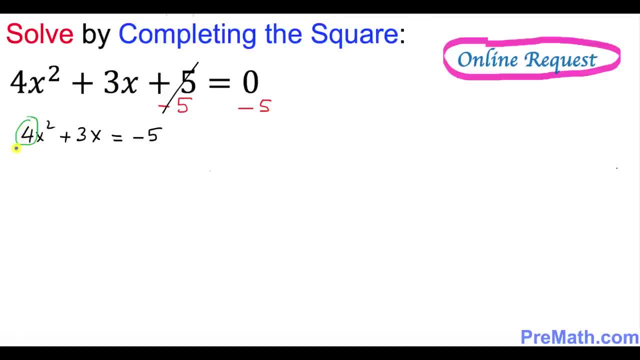 over there it is 4, so we're going to divide this one by 4. if you divide this one by 4, you must divide across the board each and every term. all right, so what we got is: 4 over 4 becomes simply 1x square plus 3 over 4x, equal to. 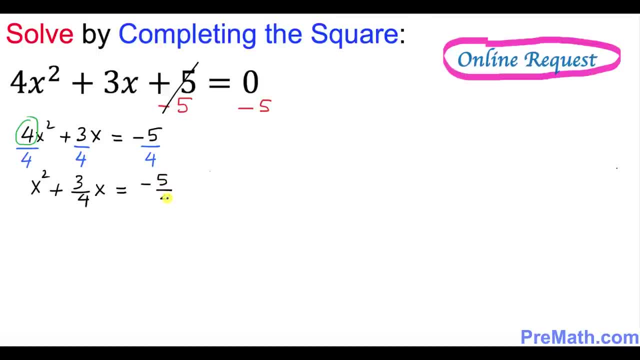 negative: 5 over 4. so the next thing, what I want you to just look at the coefficient of X, which is 3 over 4x over 4. don't worry about this sine positive sign, we are just interested in 3 over 4. I want you to put it somewhere here: 3 over 4. now I want you to divide. 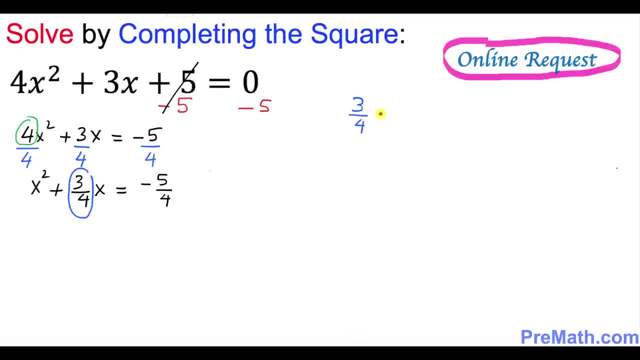 it by 2. dividing by 2 is same as multiplying by 1 over 2. so far, so good. so if you do this thing, on the top, 3 times 1 is 3, divide by 2 by 4 times 2, at the bottom is 8. so far, so good. and the next thing, what I want: 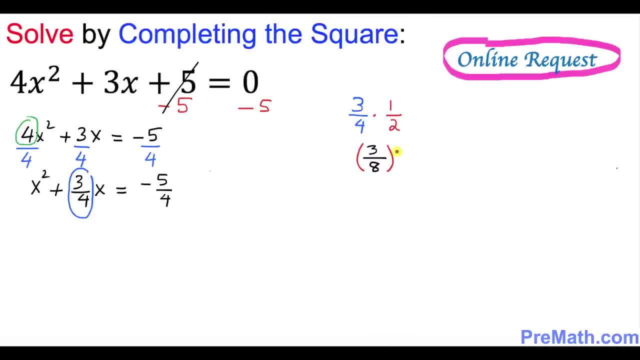 you to do is: whatever you got this thing, you must square it. so whatever this quantity we got, we're going to add it on the both sides of this equation. let's go ahead and take care of that step. so I'm going to put down x square plus 3 over. 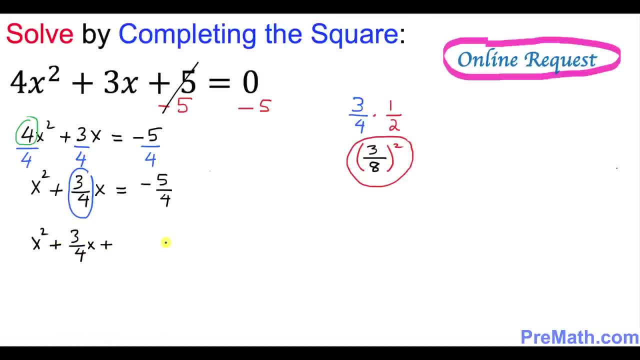 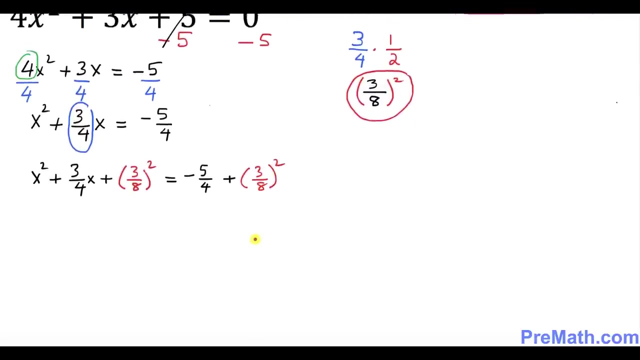 4 X plus. and then I want you to put down negative: 5 over 4 plus. now I want you to put down this: 3 over 8 square on this side and 3 over 8 square on this side as well. now look at the left hand side. 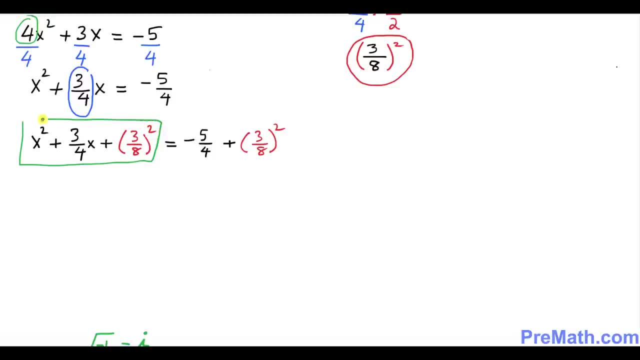 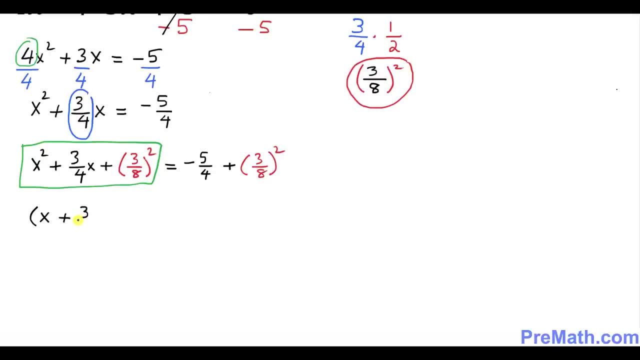 over here in this box. this represents a complete square of X plus 3, over 8 square. and now you might be wondering where this, these numbers, came from. this X came over. it showed up over here, and now you might be wondering where this numbers came from. this, these numbers came from this. these numbers came from this. 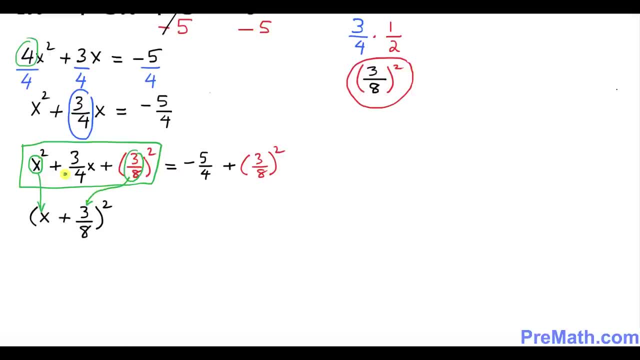 over here. this 3 over 8 showed up over here and this, whatever positive sign- this showed up over here and this is equal to just go ahead and take care of this thing. this is negative: 5 over 4 and when you square this thing, that's going. 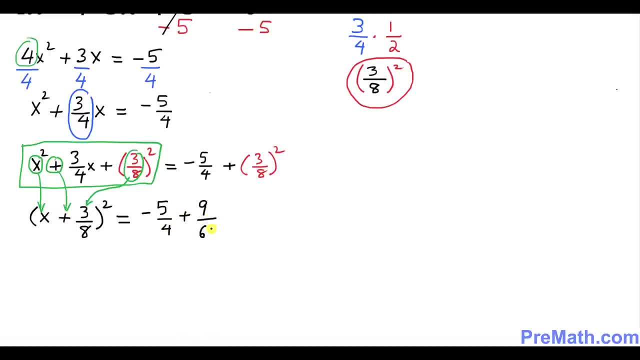 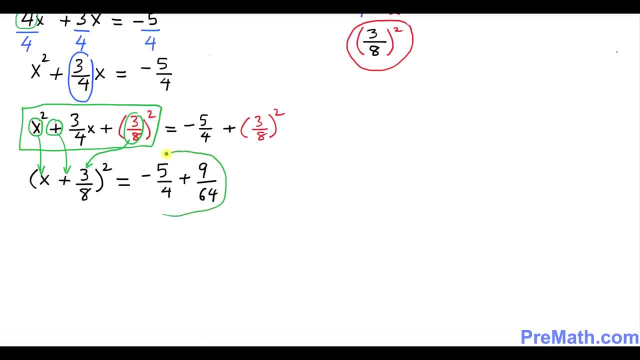 to become 9 over 64. now let's square and take care of this one, this, these two fractions we're gonna. I want you to put it somewhere here, so I put down these two fractions right up here: negative 5 over 4 plus 9 over 64- and look at these. denominator one is for 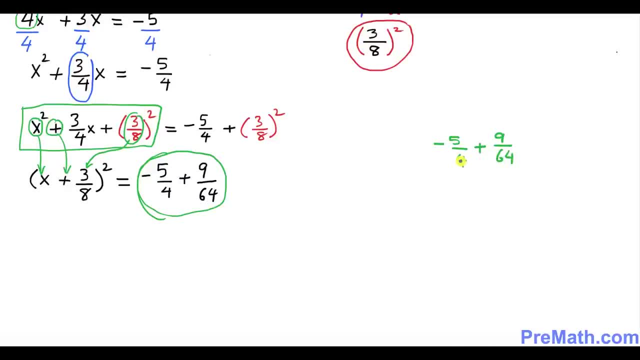 the other 164. we want to make the same denominator. so we're gonna make this for 64 by multiple. so that's the first thing we're going to do. so we're going to go by multiplying and dividing by 16. so if you multiply and divide by 16, the top 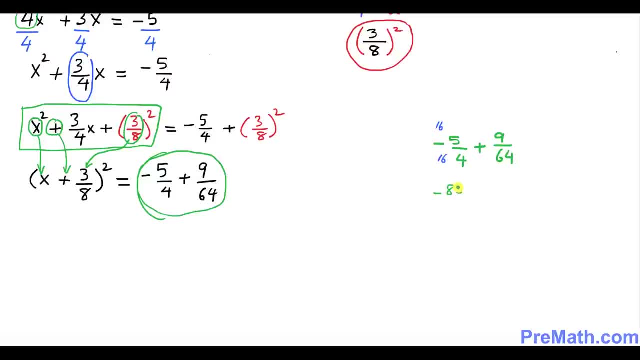 become negative 16 times 5 is 80 over 64 plus 9 over 64. since we got the same denominator, you just put it once negative 80 plus 9 turns out to be a negative 71 over 64, so I'm gonna go ahead and put down this thing over here. 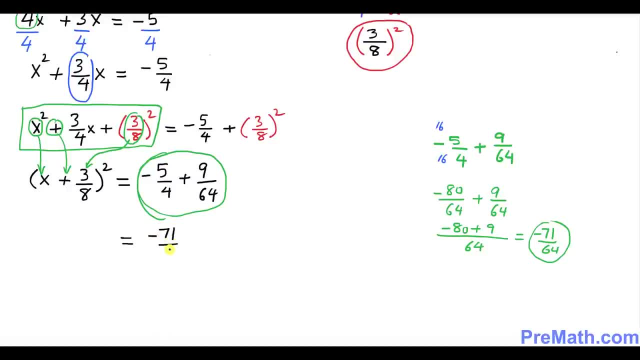 negative, 71 over 64, and on the left hand side we have a X plus 3 over 8 square. now we want to solve for X, we want to undo this square, so we're gonna take the square, our square root on both sides. take the square root on this side and take the. 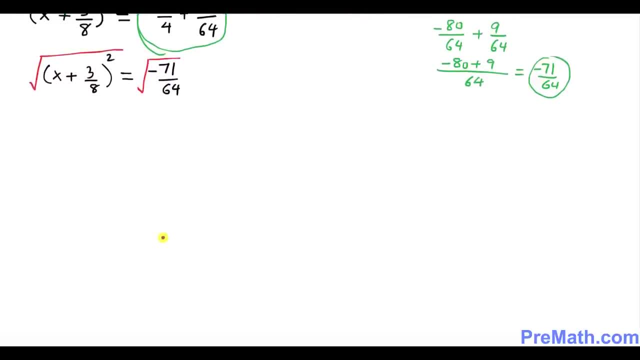 square root on this side as well. so now over here, as you can see this, this square and square root, they undo each other. so we got X plus 3 over 8 turns out to be a positive or negative, and here I can split it off. I can put square root of: